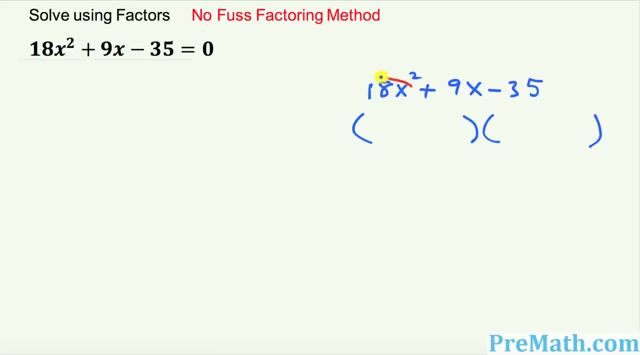 Next step: I want you to just put down this part: only: 18 X, 18 X, 18 X. do not write this exponent, just simply disregard this exponent. so we will be just put it down: 18 x right up here and 18 x right up here. next step: i want you to multiply these and numbers. 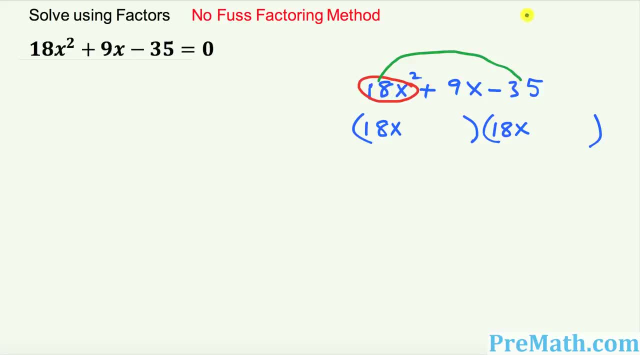 which is what? 18 and 35. i want you to write down just these 18 and 35 right up here: 18 times 35. you can multiply these ones and then you can factor them out to get this nine. right now, you can see this. we need a positive nine in the middle. but the simple way i want you to do, like 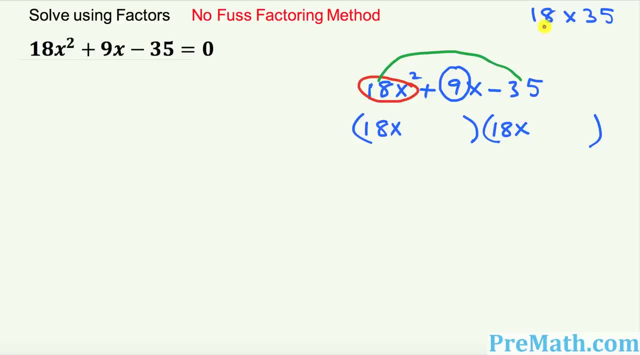 this way. okay, i want you to just manipulate this number like this thing: 18 could be factored out to what three times what six and thirty five could be factored out to what five times six, seven, isn't it now? what is the next thing i want you to do is go ahead and multiply. 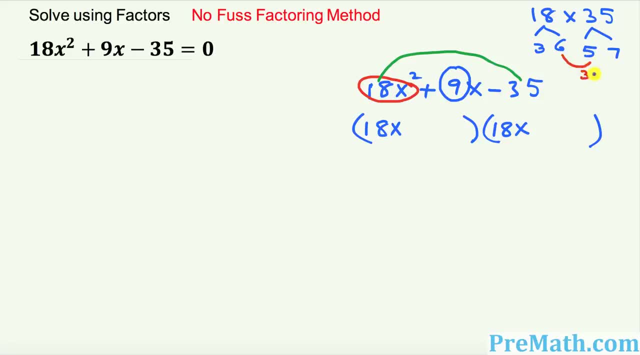 five times six, which is what 30, and three times seven is gonna give you what 21.. see, right now we got what 30 and 21. if you subtract, we're gonna get what nine. since we have a positive nine, i'm gonna make positive 30 and negative 21, so i want you to put down these: 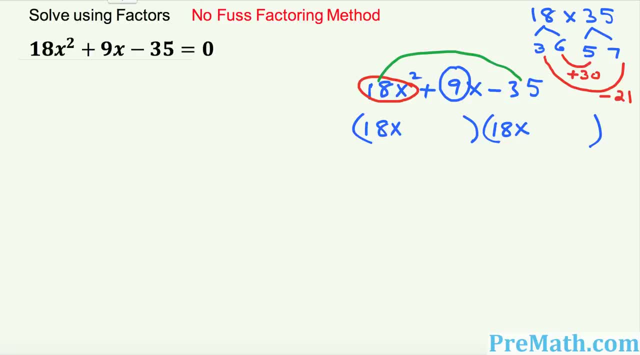 positive 30 and negative 21 right up here. so positive 30 is gonna go right up here and minus 21 is gonna go right up here. your next step is going to be this one: ask yourself in the first parentheses what is the great difference between the first and the second step. 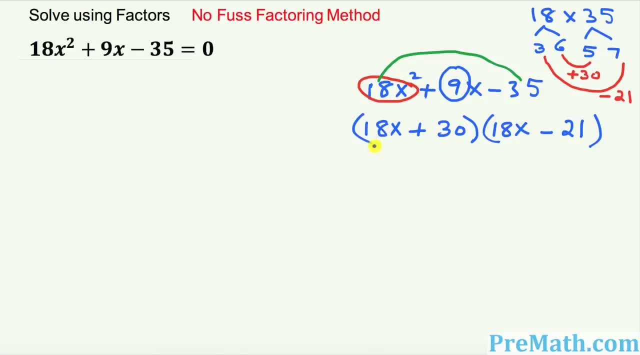 greatest common divisor, GCD. What is the biggest number that divides into both of them? So that is going to be, of course, that is going to be what, And that is going to be 6, isn't it? And look at. 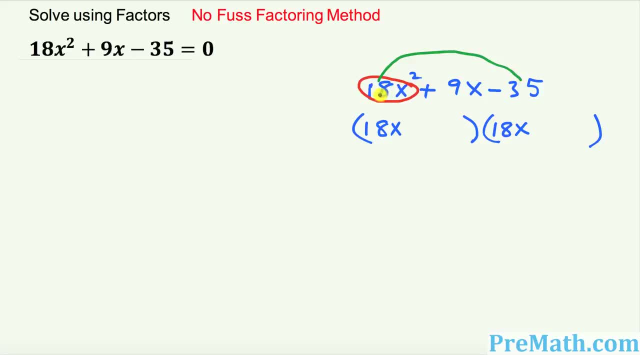 to multiply these and numbers, which is what? 18 and 35.. I want you to write down just these 18 and 35 right up here: 18 times 35.. 18 times 35. You can multiply these ones and then you can factor them out to get this 9 right. 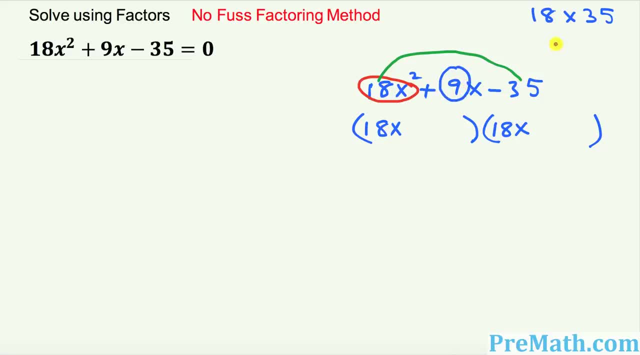 now You can see this. we need a positive 9 in the middle. But the simple way I want you to do, like this way, okay, I want you to just manipulate these number like this thing: 18 could be factored out to what 3 times what 6 and 35 could be. 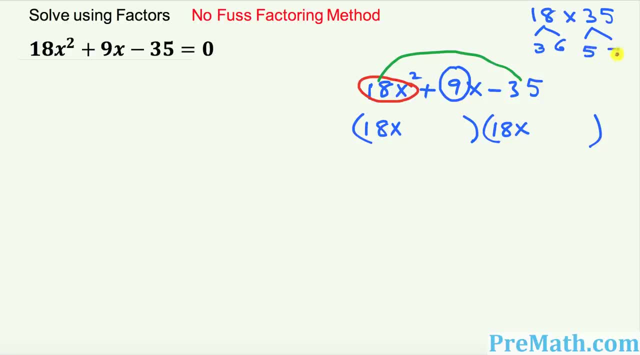 factored out to what 5 times 6. 7, isn't it? Now, what is the next thing I want you to do is go ahead and multiply 5 times 6, which is what 30 and 3 times 7 is. 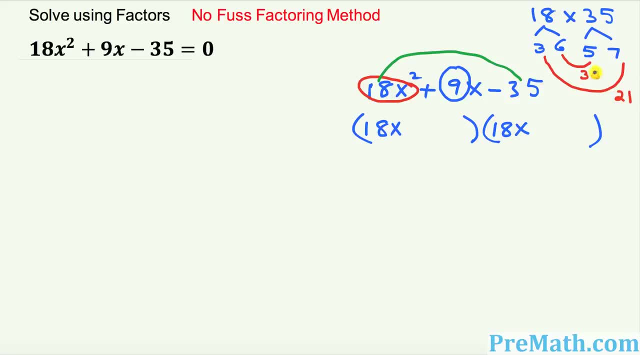 gonna give you what 21.. See, right now we got what 30 and 21. if you subtract, we're gonna get what 9.. Since we have a positive 9, I'm going to make positive, positive 30 and negative 21, so I want you to put down these positive 30 and. 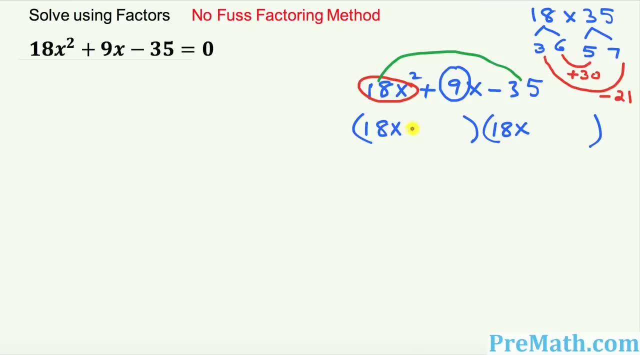 negative 21 right up here. so positive 30 is gonna go right up here and minus 21 is gonna go right up here. your next step is going to be this one: ask yourself in the first parentheses what is the greatest common divisor? GCD are which. 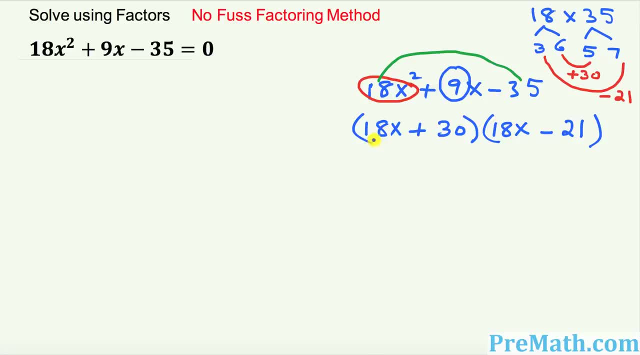 what is the biggest number that divides into both of them. so that is gonna be, of course, that is gonna be what? and that is going to be 6, isn't it? and look at this thing: you tell me what numbers they're gonna divide by this one and, yes, the. 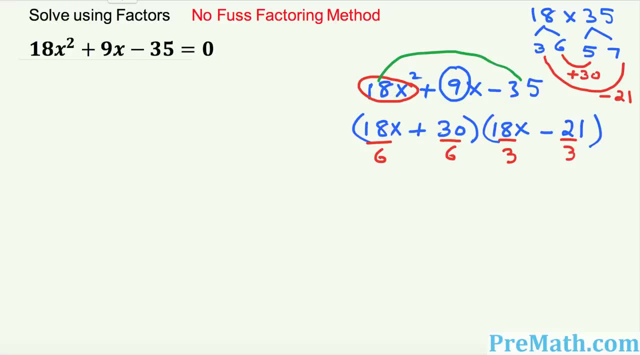 biggest number is 3. that's right. and now, finally, one more thing I want you to do. is you want to do, is you want to divide the? once you do this thing, 6 goes into 18. what 3 times? so 3x plus 5 times this. 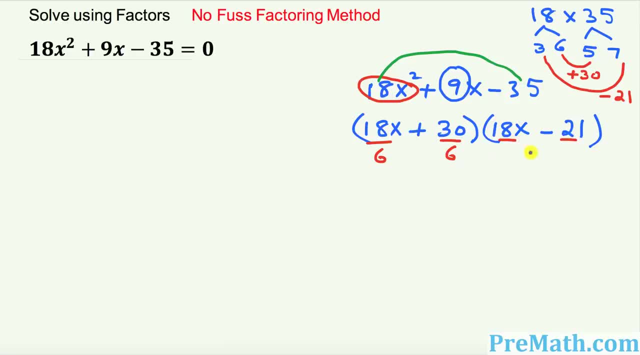 this thing. You tell me what numbers they're going to divide by this one, And, yes, the biggest number is 3.. That's right. And now, finally, once you do this thing, 6 goes into 18. what 3 times So 3x. 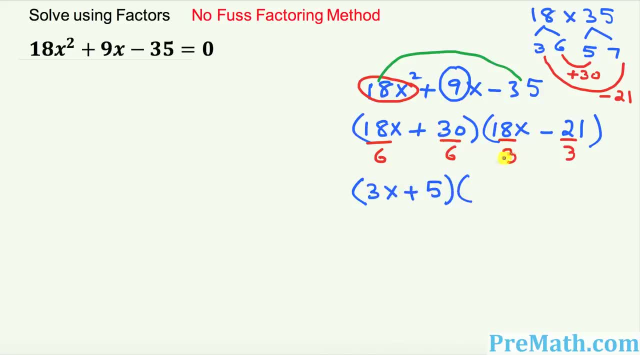 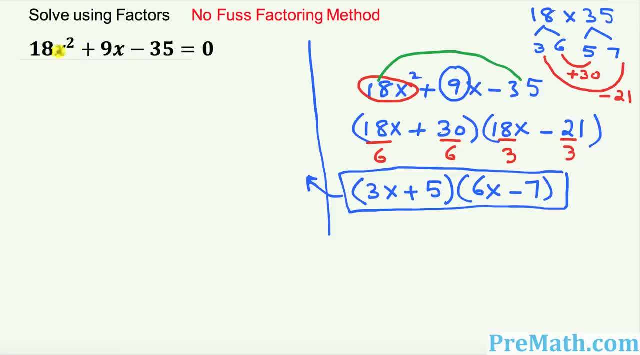 to put this one here, And I want you to put this one here, And I want you to put this one here And then put this back right up here. So these, right now the left-hand side- I can put over here these. 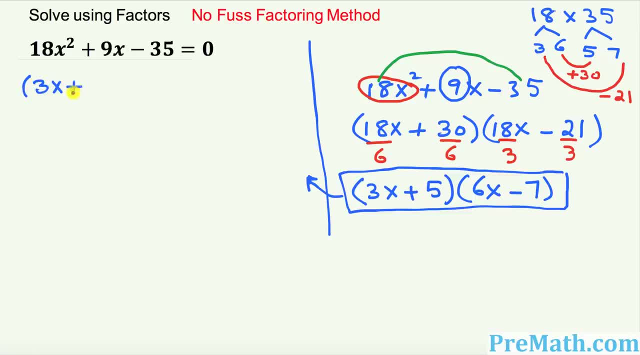 factors, which is what? 3x plus 5 times 6x minus 7, that is equal to 0.. So once we have taken care of this one, now, since we have a 2 parentheses, they are multiplying And that is equal to 0.. We can. 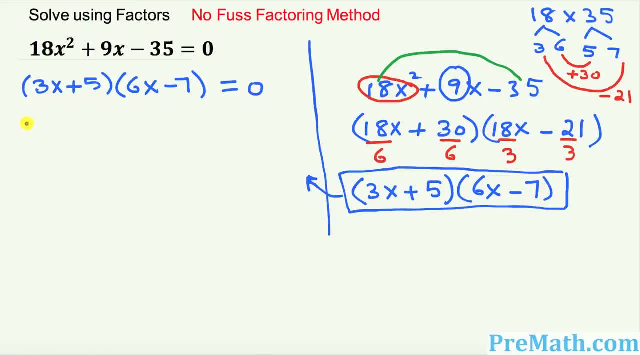 break them down. We can do this thing. This is the biggest thing that divides into both of them down. we can write them as a two separate equations. the first equation is going to be 3x plus 5, equal to 0, and the second equation, on this side, is going to be 6x. 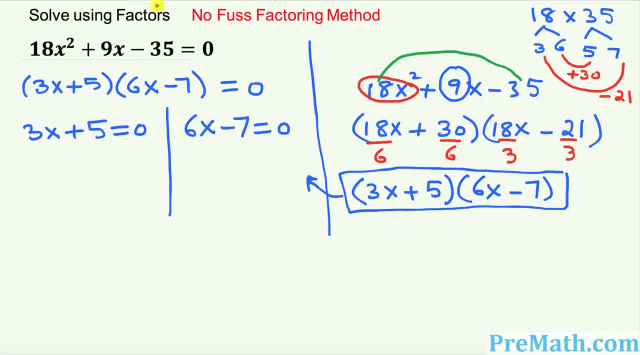 minus 7, equal to 0. let's go ahead and solve for X on both side. that means we're going to isolate X. so first I want you to subtract 5 from both side. this is gone. so what we got right now we got 3x, equal to what negative 5? now I want you. 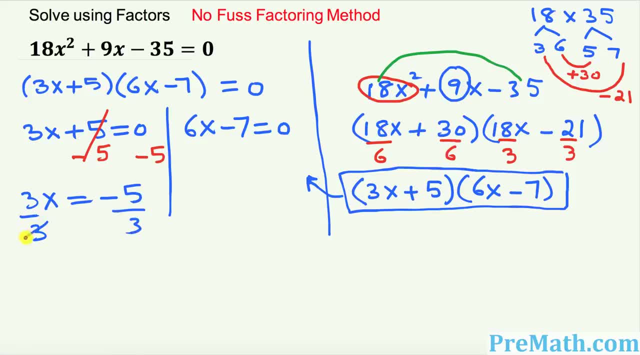 to divide both side by 3. this 3 and 3 is gone. so X equal to negative 5 over 3 is one of our solution to this quadratic equation. likewise, we're going to do the same process over here, since this is negative 7. so we: 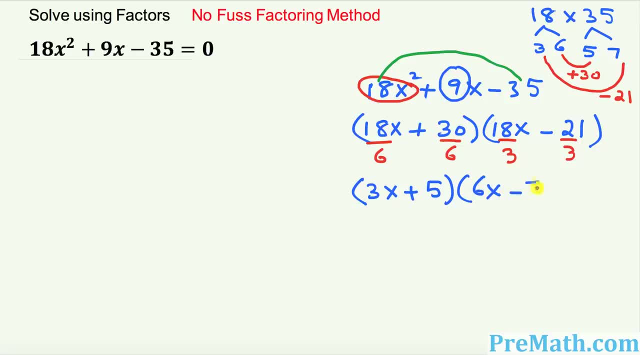 simply become what 6x minus what 7, and that turns out to be the factors of our this quadratic polynomial. so once we have done these one, I want you to put this one back right up here. so these, right now the left hand side, I can put over here these factors, which is what. 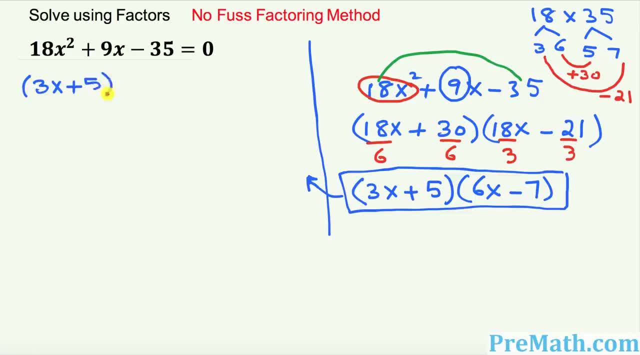 3x plus 5 times 6x minus 7, that is equal to 0. so once we have taken care of care of these one now, since we have a two parentheses, they are multiplying and that is equal to 0. we can break them down, we can write them as a two separate. 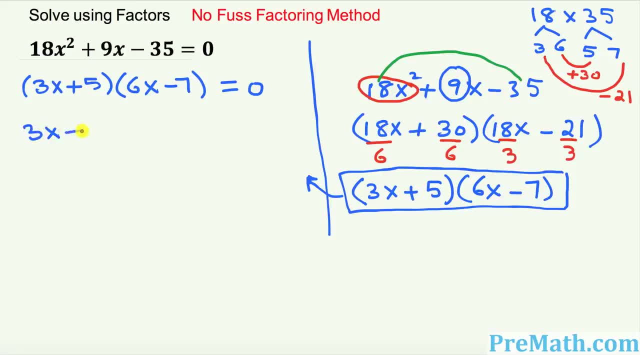 equations. the first equation is going to be 3x plus 5, equal to 0, and the second equation on this side is going to be 6x minus 7, equal to 0. let's go ahead and solve for X on both side. that means we're gonna isolate X so fast. I want you. 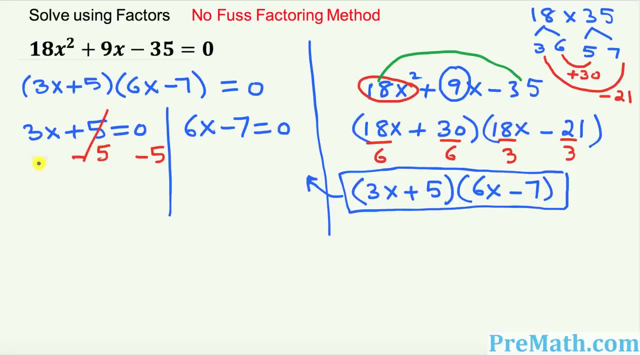 to subtract 5 from both side. this is gone. so what we got right now? we got 3x. equal to what negative 5? now I want you to divide both side by 3. this 3 and 3 is gone, so X equal to negative 5 over 3 is one of our solution to this quadratic. 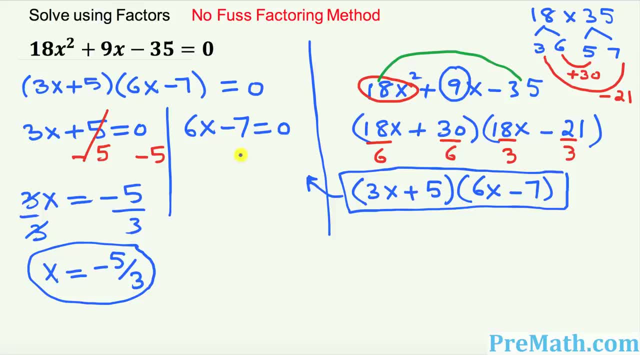 equation. likewise, we're gonna do the same process over here. since this is negative 7, so we have to add 7 on both side. this thing, what happened, this thing cancels out so what we got? 6x equals to what 7? now I want you to divide by 6 both sides this. 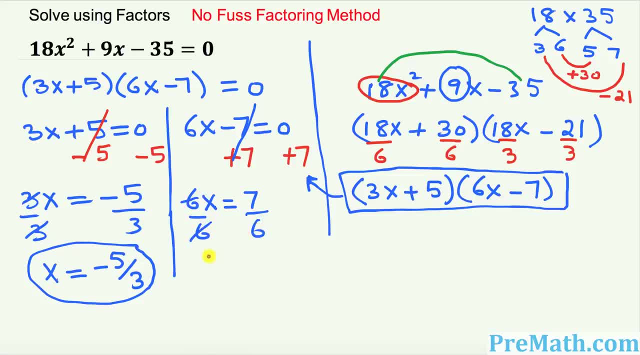 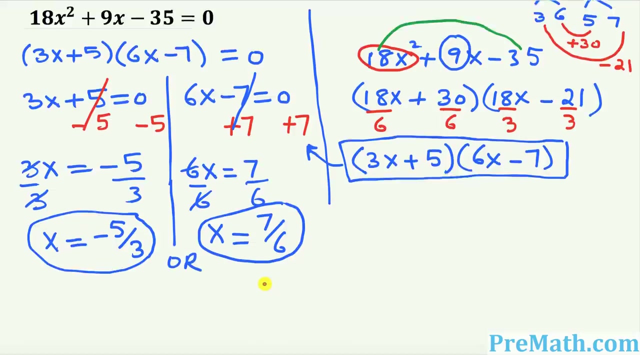 6 and 6. they cancel each other out. so X by itself equals to what 7 over 6, and that is our another solution. so thus our two solutions are: are either x equal to negative 5 over 3 or x equal to 7 over 6.. Or we can write a little bit.